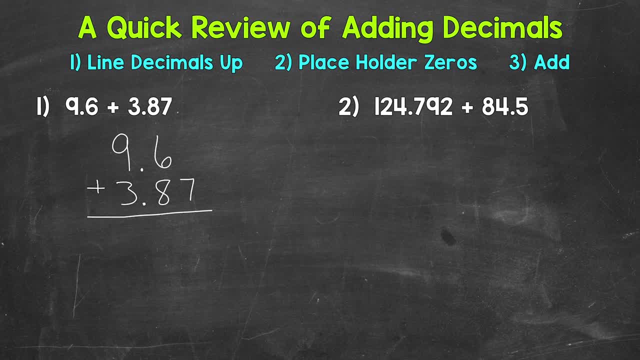 Remember, zeros to the right of a decimal do not change the value of that decimal. So, we're going to be working with an equivalent decimal. We're not changing the value of the problem at all. So, we're able to use placeholder zeros to the right of a decimal. So, let's put a zero here in the hundredths place. And now, both of our numbers go to the hundredths. And we're able to add. So, we'll start with the hundredths. 0. Plus 7 is 7. 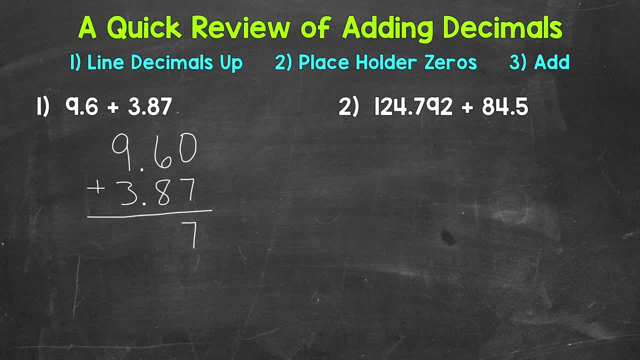 Then, we'll move to the tenths. 6 plus 8 is 14. So, we carry our 1. Now, our decimal goes straight down into our answer. It's lined up throughout the entire problem. Now, we'll move to the ones place, where we have 1 plus 9 plus 3. 1 plus 9 is 10. Plus 3 is 13. 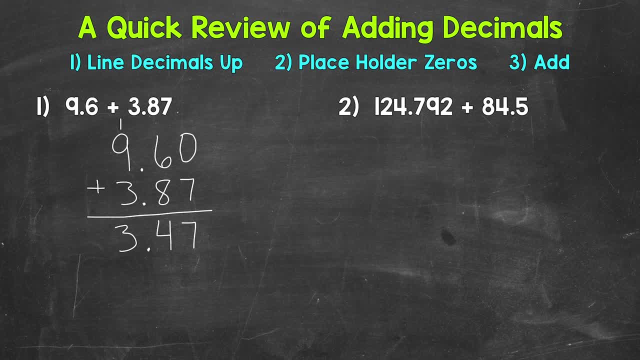 So, we'll put our 3. And then, our carried 1. We'll be brought straight down. 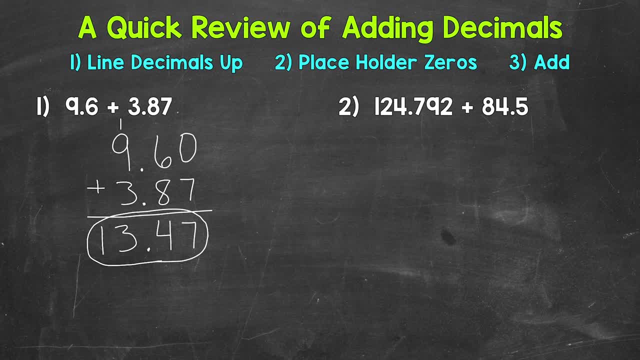 And we end up with 13 and 47 hundredths. 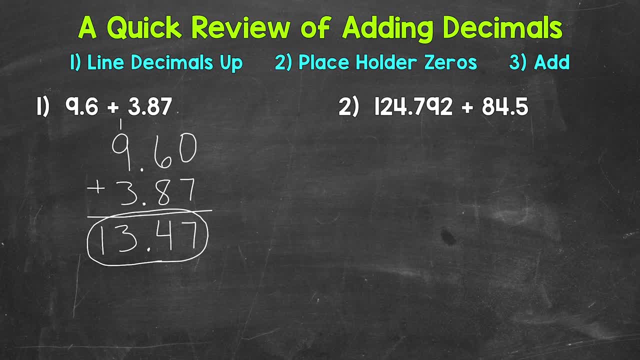 Let's move on to number 2, where we have 124 and 792 thousandths plus 84 and 5 tenths. So, let's line our decimals up here. 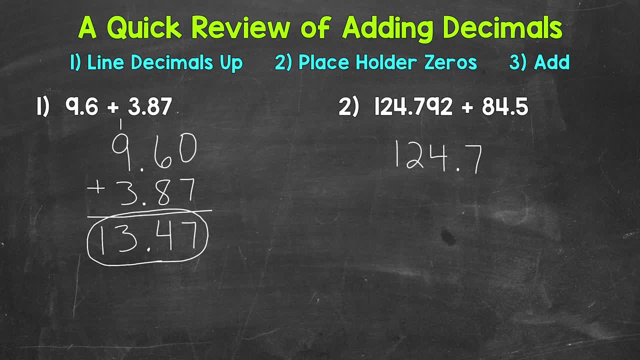 124 and 792 thousandths. 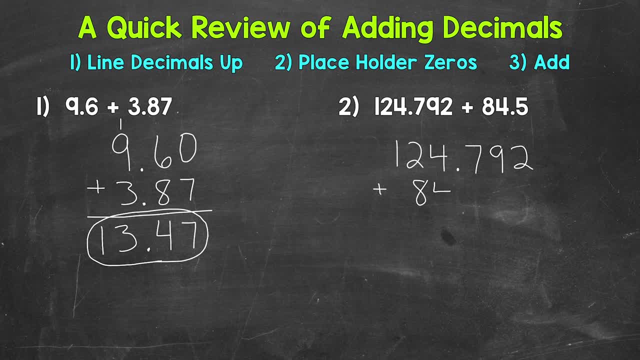 Plus. 84 and 5 tenths. 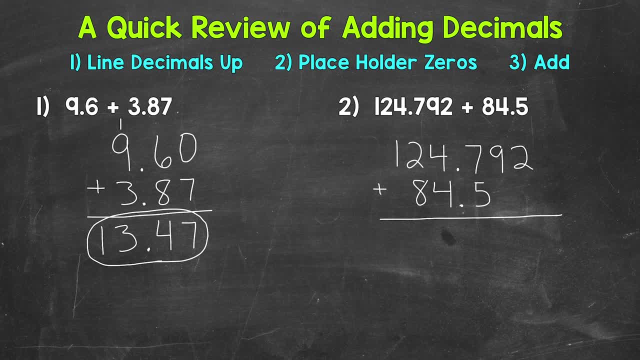 So, let's use placeholder zeros to line this up a little better here. A zero in the hundredths. And then, a zero in the thousandths. 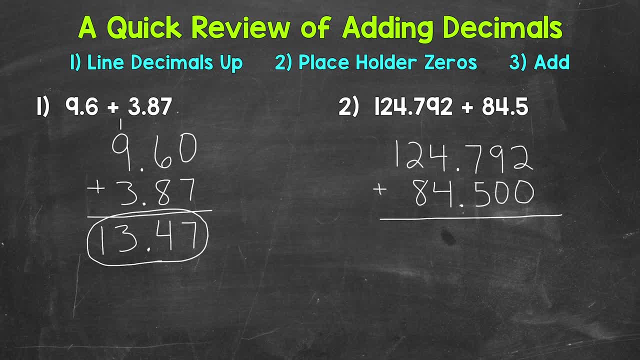 Again, zeros to the right of a decimal do not change the value of that decimal. It's an equivalent decimal. So, we're able to use those placeholder zeros. 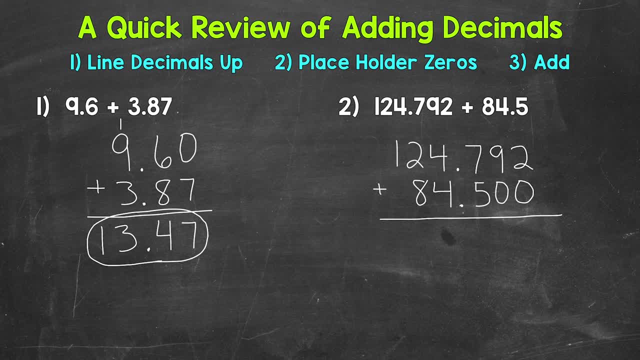 Now, we can add. So, we'll start with the thousandths place. 2 plus 0 is 2. 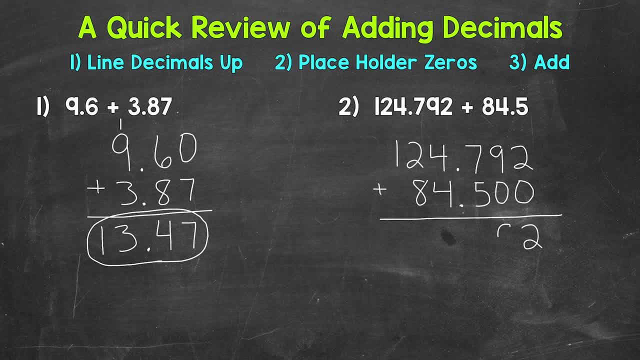 The hundredths place. 9 plus 0 is 9. The tenths place. 7 plus 5 is 12. So, we'll put our 2. And then, carry the 1. We can bring our decimal straight down into the answer. Now, we have the ones place. 1 plus 4 is 5. Plus 4 is 9. The tens place. 2 plus 8 is 10. So, we'll put our 0. 0 here. Carry the 1. 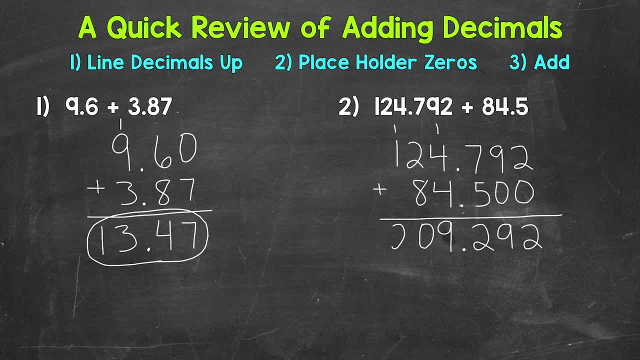 And then, the hundredths place. 1 plus 1 is 2. 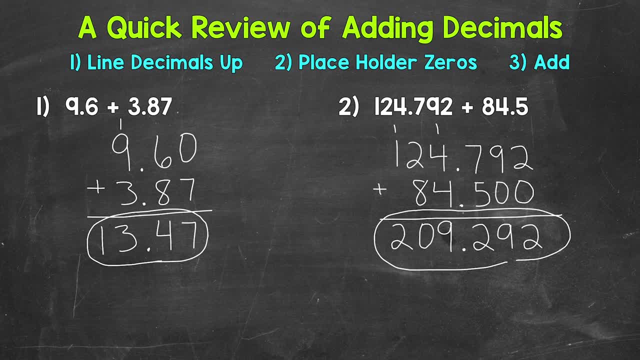 So, we end up with 209 and 292 thousandths. That's how we add decimals. Let's move on to subtraction. 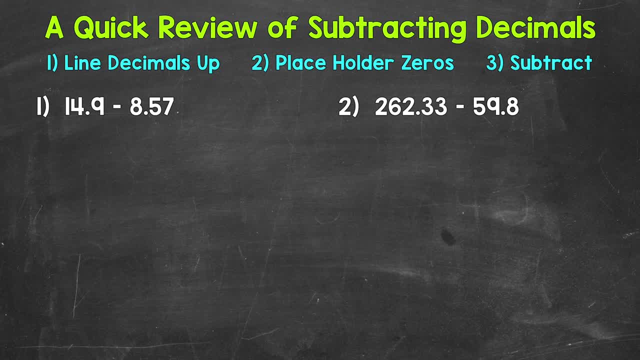 So, here are our examples of subtracting decimals. Let's jump into number 1, where we have 14 and 9 tenths. Minus. Minus 8 and 57 hundredths. Now, just like when we add decimals, when we subtract decimals, we need to line the decimals up. That's going to line up all of our places. So, let's rewrite this first problem vertically here, lining up the decimals. 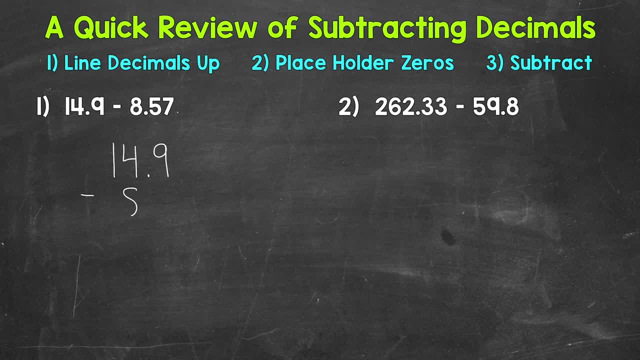 So, 14 and 9 tenths minus 8 and 57 hundredths. So, the decimals are lined up. And that's going to line up all of our places. Now, that problem looks a little offset because 14 and 9 tenths goes to the tenths place. And then, 8 and 57 hundredths goes to the hundredths place. So, just like when we add decimals, we can use placeholder zeros to have this look more lined up. So, let's use a placeholder zero in the hundredths place here. And then, both of our decimals go to the hundredths place. Remember, zeros to the right of a decimal. 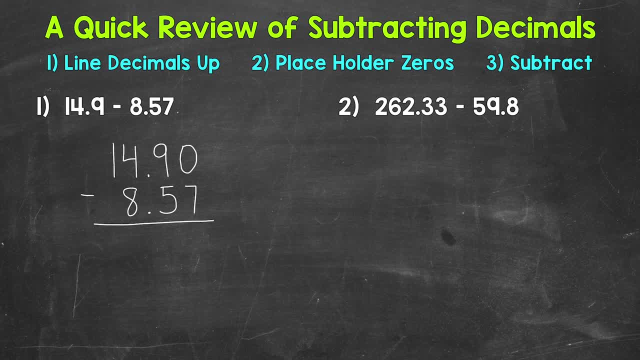 If you have a decimal, do not change the value. That's an equivalent decimal and does not change the value of the problem at all. 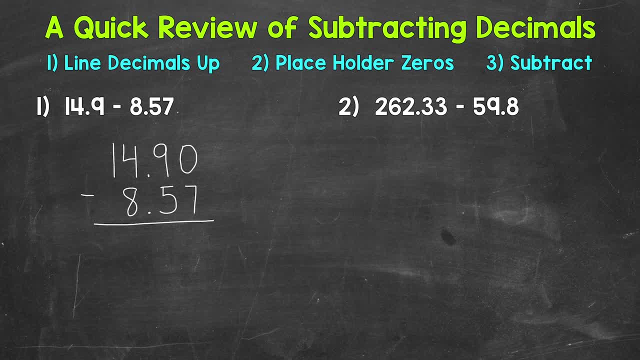 Now, we're able to subtract. So, we'll start with the hundredths place. We have 0 minus 7, which we need to borrow. So, let's borrow from the 9. That's an 8 now. And we have 10 minus 7, which is 3. Then, we move to the tenths place. 8 minus 5, 3. 3. 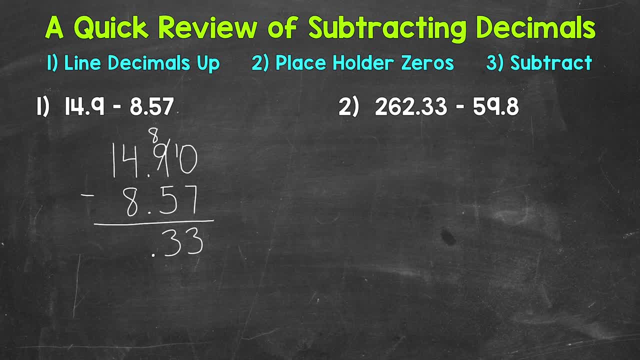 4 decimal straight down into the answer. The decimal is lined up throughout the entire problem. 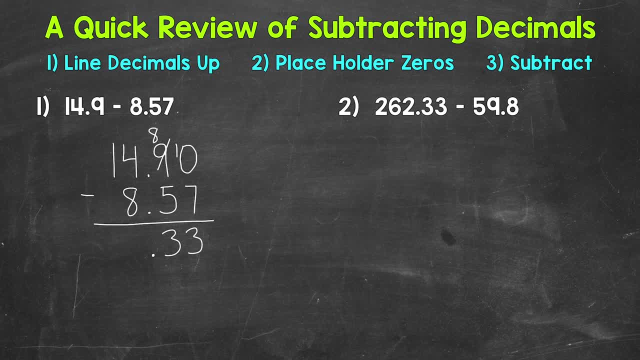 Then, we move to the ones place. 4 minus 8. We need to borrow from the tens place here. So, that's a 0. And that's a 14. 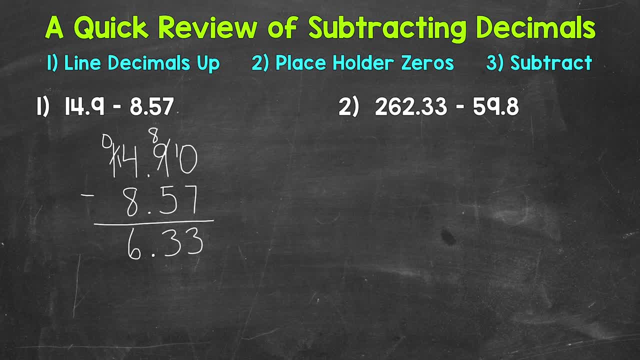 So, 14 minus 8 is 6. And we are done. 6 and 33 hundredths. 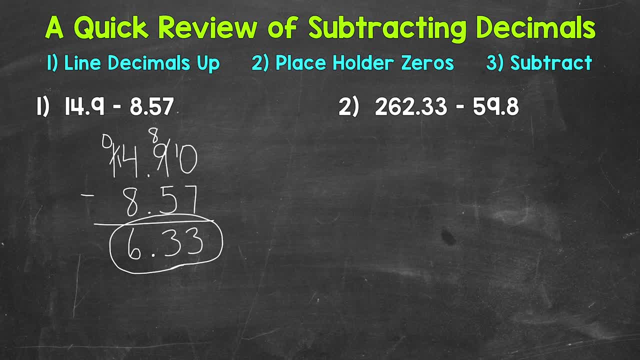 Now, I do want to mention one more thing before moving on to number 2. And this is going to be a common mistake. That you'll want to avoid. 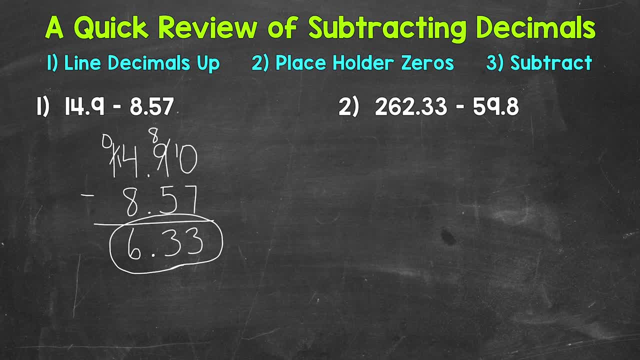 And using placeholder zeros will actually help you avoid this mistake. So, let me rewrite the problem here real quick to the side. 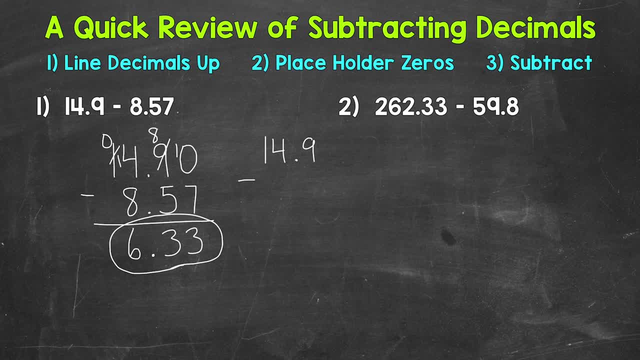 So, we have 14 and 9 tenths minus 8 and 57 hundredths. 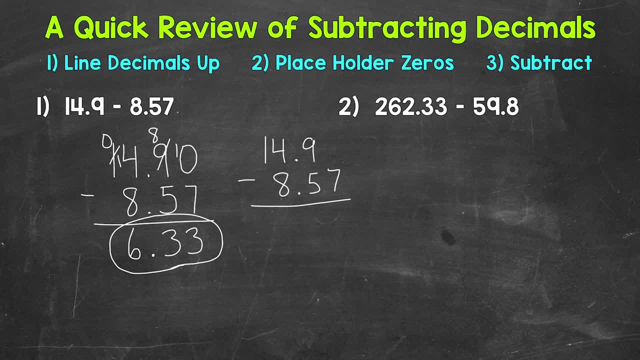 So, dropping the 7. So, starting with the hundredths place. And then, just dropping the 7 because there isn't anything above it is not correct. 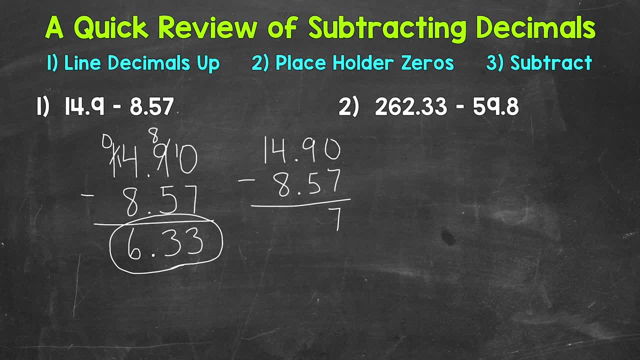 We actually have 0 minus 7 there. So, we needed to borrow. And you can see, we do not have a 7 in the hundredths place in our final answer. So, again, avoid the mistake of just dropping that number. Because, really, we have 0 minus 7 there. And we need to borrow. So, be careful of that. 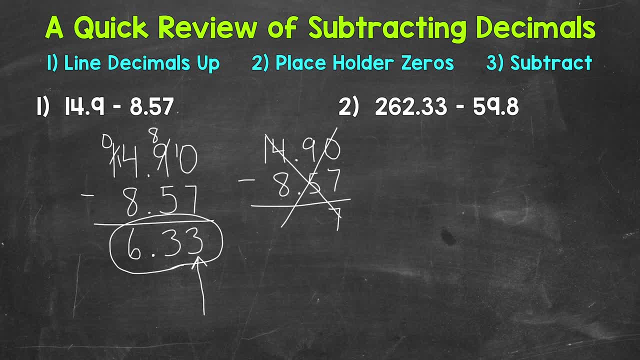 Let's move on to number 2 where we have 262 and 33 hundredths. Minus. Minus 59 and 8 tenths. So, we will start by lining up our decimals here. So, 262 and 33 hundredths minus 59 and 8 tenths. We can use a placeholder zero. So, these both go to the hundredths. And now, we are able to subtract. So, we'll start with the hundredths. 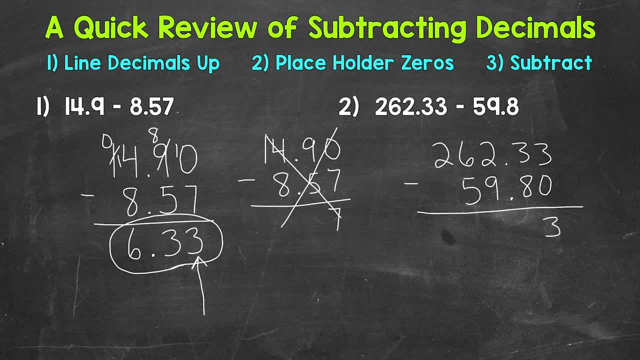 3 minus 0 is 3. The tenths. The tenths place. 3 minus 8. Well, we need to borrow. So, borrow from the 2. That's a 1. And we have a 13. So, 13 minus 8 is 5. 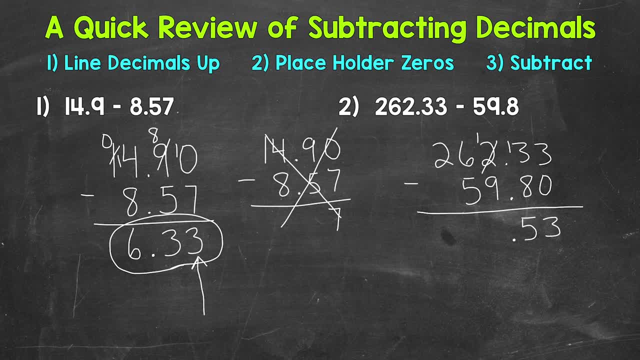 We can bring our decimal straight down into our answer. And now, we have the ones place. So, 1 minus 9, we need to borrow. So, we'll borrow from the 6. And we have 11 minus 9, which is 2. Then, for the tens place, we have 5. 5 minus 5, which is 0. And then, lastly, we have the hundreds place, where we have 2 minus nothing under it. So, it's just 2 minus 0, which is 2. Now, that's how we subtract decimals. Let's move on to multiplication. 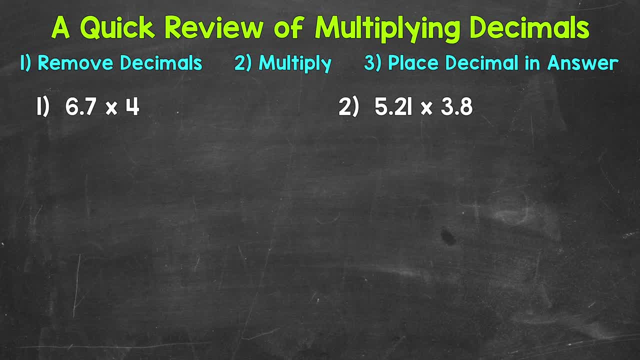 Here are our examples of multiplying decimals. Let's jump into number 1, where we have... 6 and 7 tenths times 4. 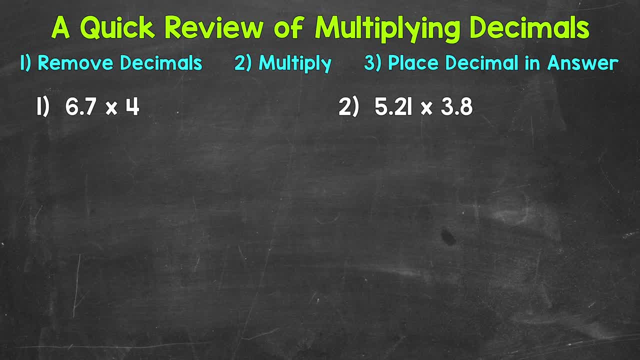 Now, the first thing that we're going to do when we have a multiplication problem that involves decimals, we're going to remove any decimals within the problem. 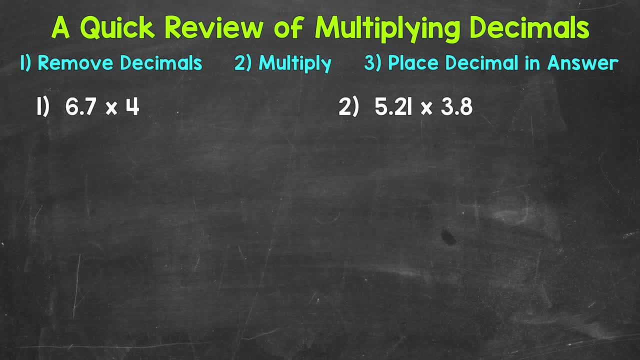 So, we're going to multiply just like we would if we had whole numbers. 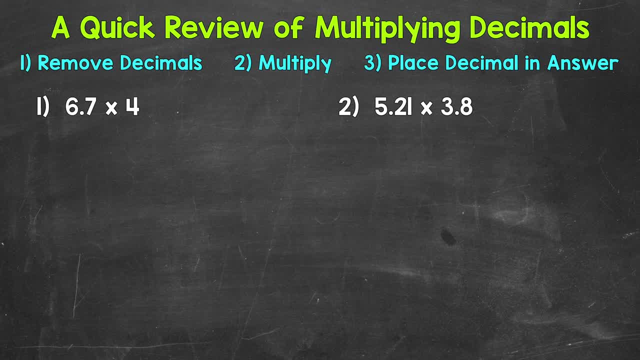 Let's set this up and rewrite number 1 as 67 times 4. So, again... Remove any decimals. We're going to worry about placing the decimal in our answer once we multiply. So, once we remove the decimals, we can multiply. So, we'll start with 4 times 7, which is 28. So, carry that 2. And then, we have 4 times 6, which is 24, plus that 2 is 26. 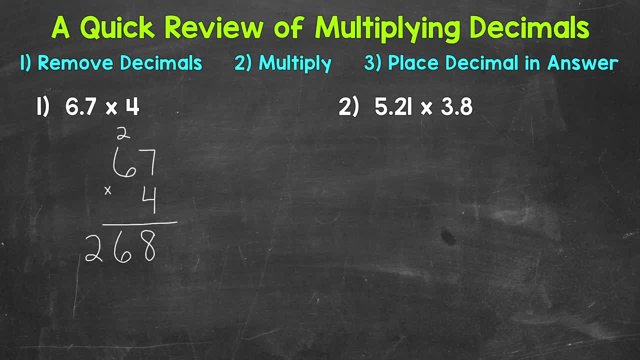 Now, we're done multiplying. So, we... We can place our decimal in our answer. 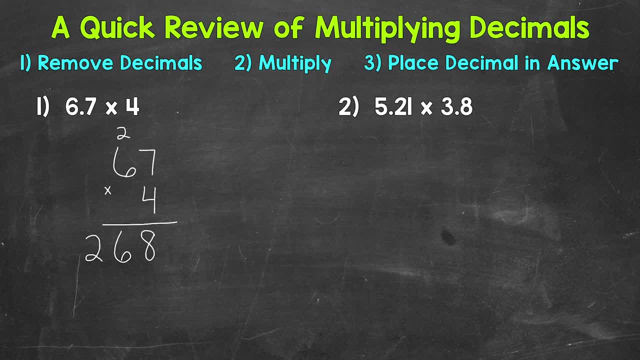 So, we take a look at the original problem and see how many digits are behind or are to the right of a decimal. Well, 1. We have this 7 right here to the right of a decimal. So, our answer is going to have one digit to the right or behind the decimal. So, one digit would be this 8. So, we can place our decimal in between. The 6 and the 8. 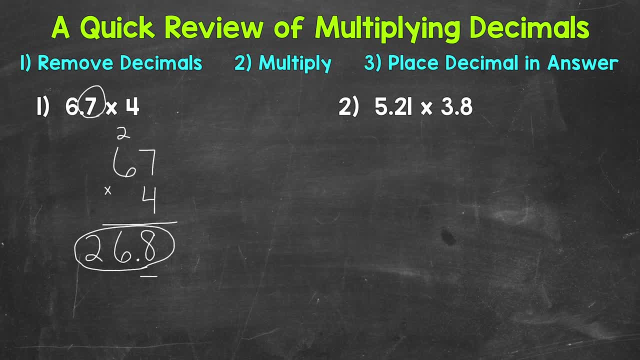 Our final answer, 26 and 8 tenths. 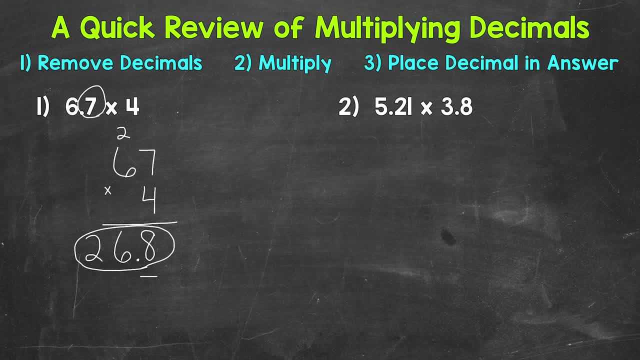 Let's move on to number 2, where we have 5 and 21 hundredths times 3 and 8 tenths. 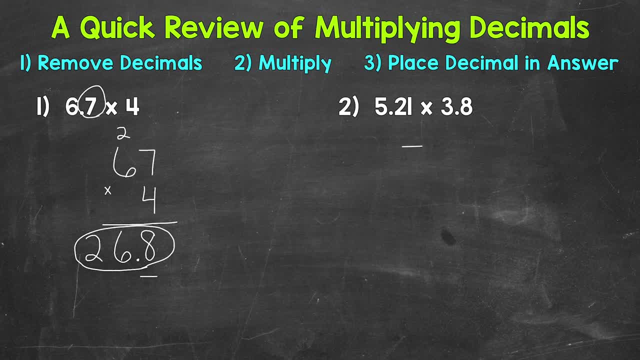 So, let's remove the decimals and rewrite this problem. So, 521 times 38. 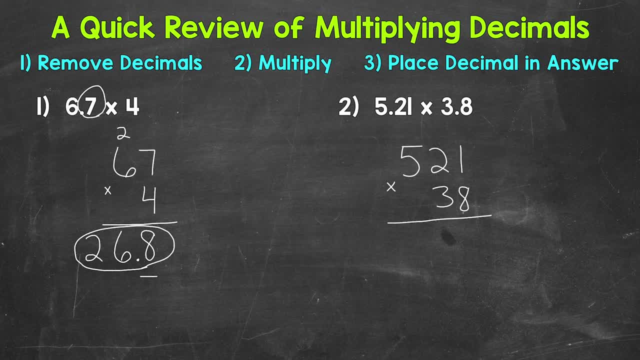 Now, we're ready to multiply. So, 8 times 1 is 8. 8 times 2 is 16. Put our 6, carry the 1. 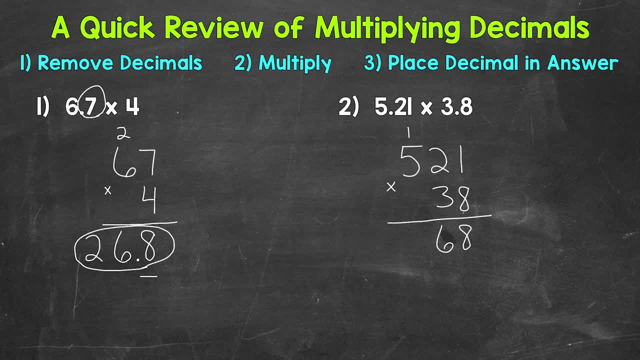 And then, 8 times 5 is 40, plus that 1 is 41. 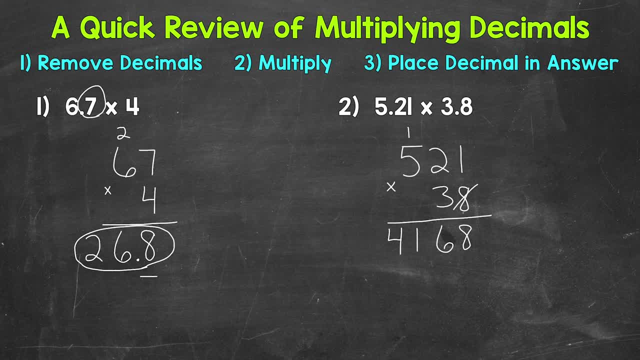 So, we are done with the 8, and we are done with this carried 1. So, we're going to move over to the 3. We're moving one place value to the left. So, we need our placeholder 0 here. And now, we multiply, starting with 3 times 1, which is 3. 3 times 2 is 6. And then, 3 times 5 is 15. Now, we add. 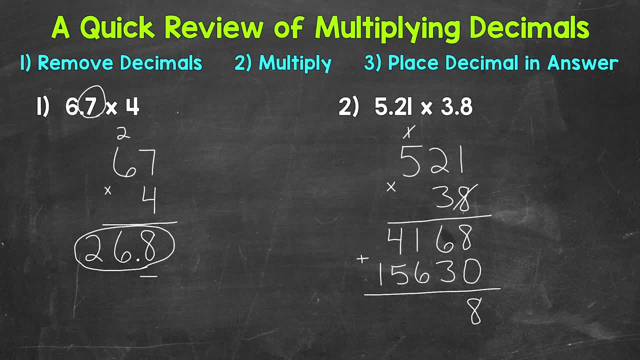 So, 8 plus 0 is 8. 6 plus 3 is 9. 1 plus 6 is 7. 4 plus 5 is 9. 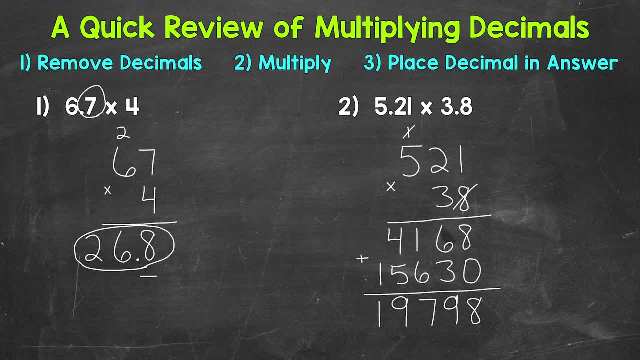 And then, we have a 1. So, once we get to this point, we look at our original problem and see how many digits are to the right or are behind a decimal. Well, this 2 would be 1, this 1 would be 2, and then this 8 would be 3. So, we have 1, 2, 3 digits behind or to the right of a decimal. 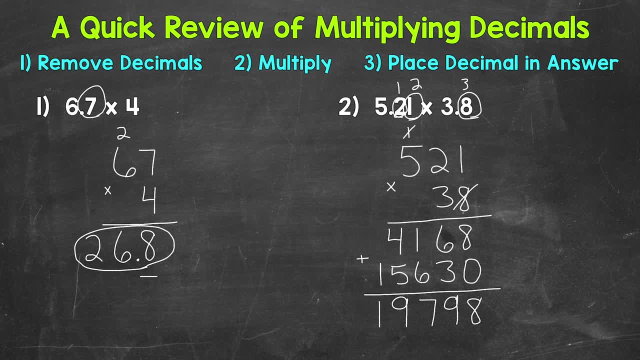 So, our answer needs 3 digits to the right of the decimal. So, we have 1. 2. 3 digits. 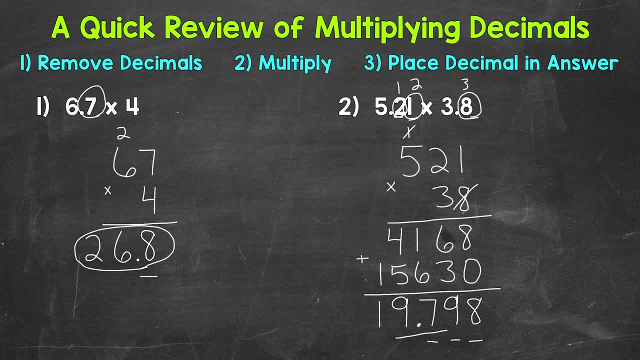 Our decimal is going to go between the 9 and the 7. Our final answer, 19 and 798 thousandths. So, there you have it. 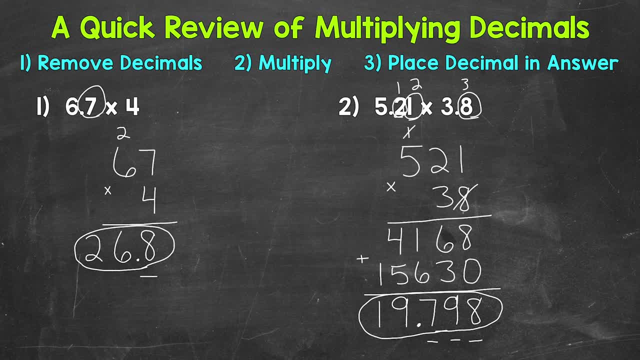 There's a quick review of multiplying decimals. Remove the decimals. 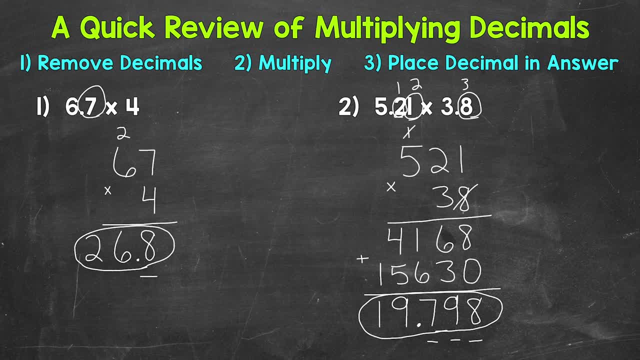 Multiply as you normally would with whole numbers. And then, place your decimal in the answer. Look at the original problem. See how many digits are. 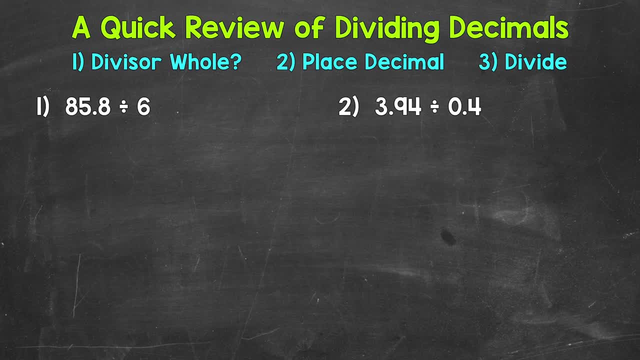 Let's move on to division. Here are our examples of dividing decimals. Let's jump into number 1, where we have 85 and 8 tenths divided by 6. Now, the first thing that we're going to do, we're going to set the problem up and place our decimal. 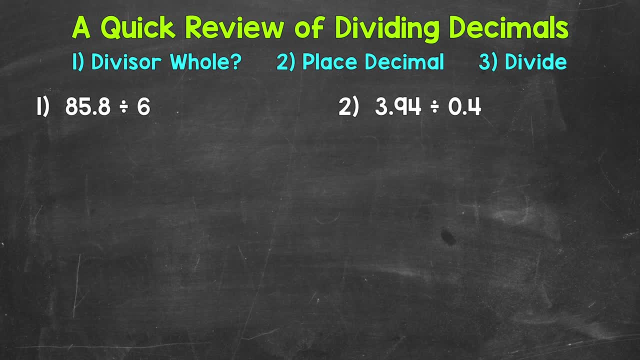 For number 1, we have 85 and 8 tenths. For our dividend. That's the number we are dividing. 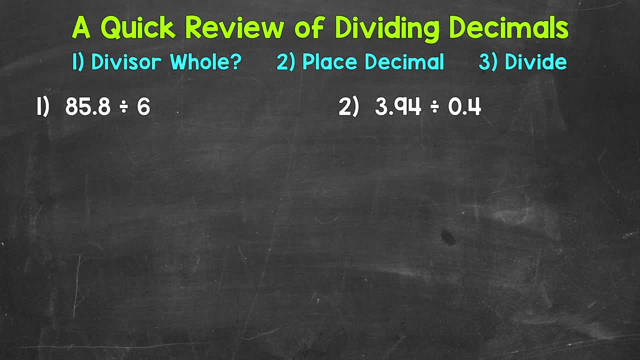 So, it goes under our division bar. So, let's write out 85 and 8 tenths. 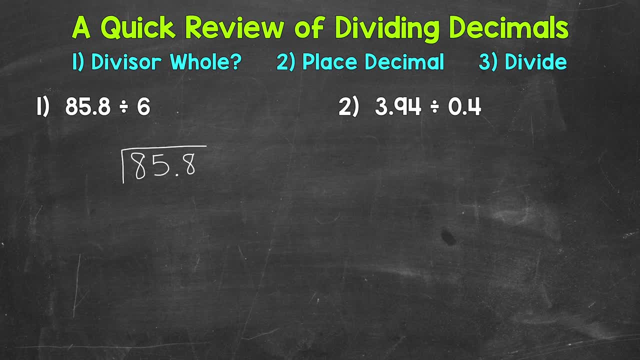 And then, we are dividing by our divisor of 6. So, the divisor is the number we are dividing by. 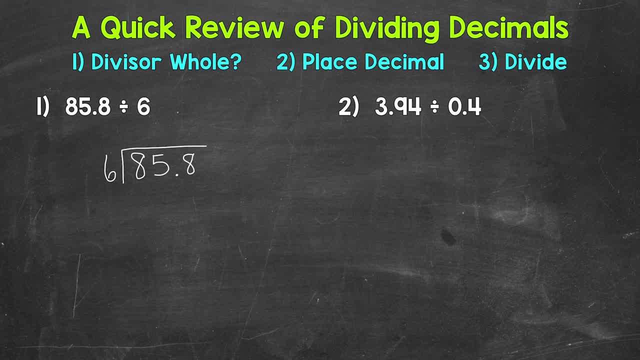 Once we get to this point and we are set up, we have a very important question. Is our divisor a whole number? If yes, our decimal goes straight up into our answer. 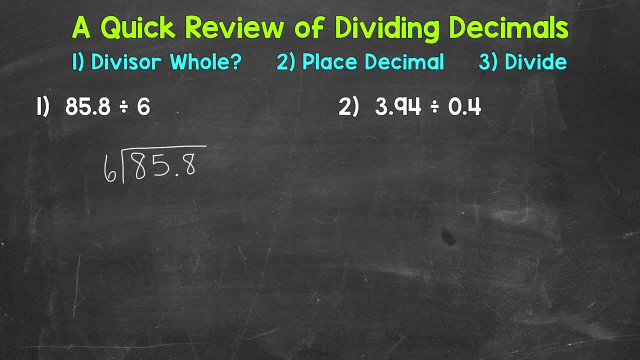 For number 1, our divisor is whole. We have a 6. 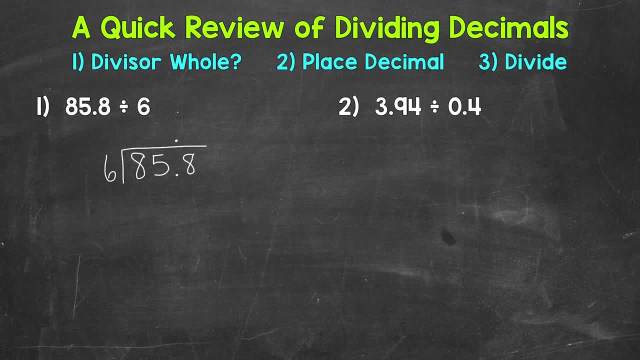 So, let's bring that decimal straight up into our answer. 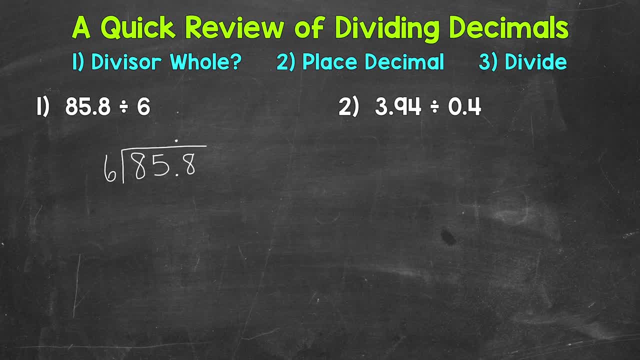 So, our decimal is placed and we are ready to move on. 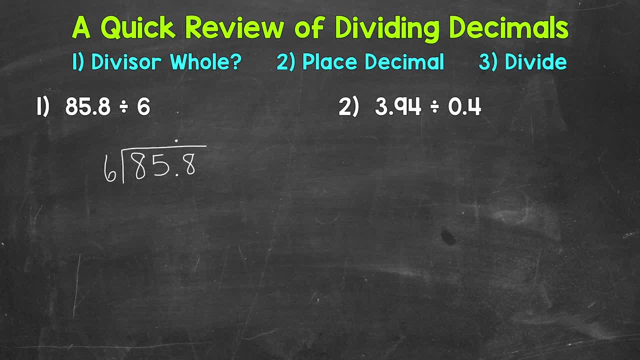 Now, I do want to mention, for number 2, we will see what happens when we do not have a whole number for our divisor. So, once we bring that decimal straight up into our answer, we can divide as we normally would with whole numbers. So, we are going to use the same division process that we use with whole numbers. Divide, multiply, subtract, bring down, repeat. So, let's start with divide. 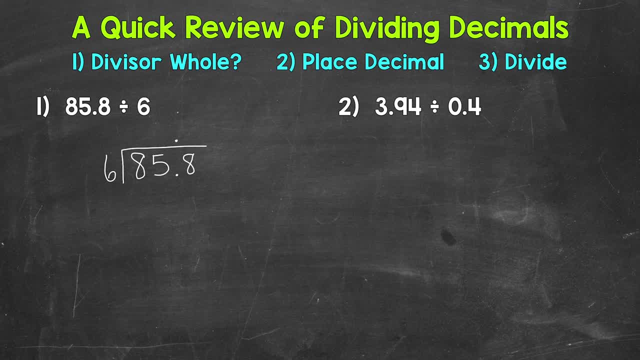 So, we have 8 divided by 6. How many whole groups of 6 are in 8? Well, 1. 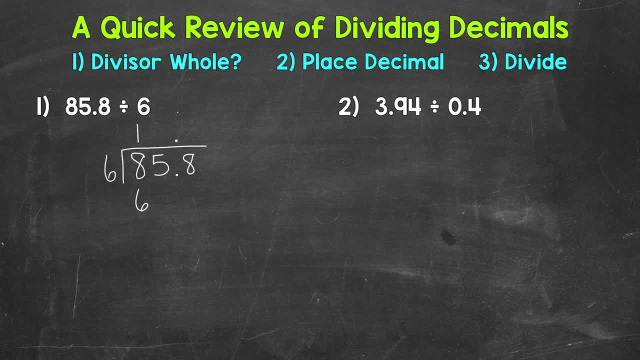 Then, we multiply. 1 times 6 is 6. Subtract. 8 minus 6 is 2. And then, we bring down. Now, we repeat. 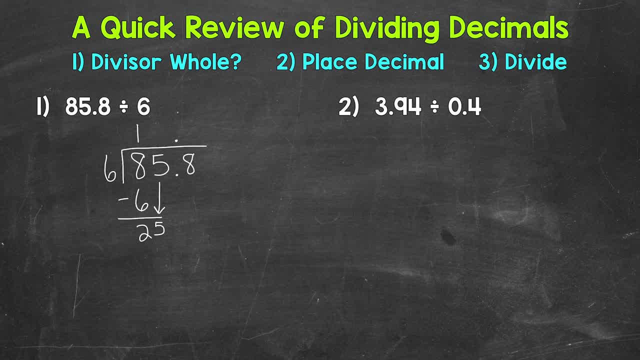 So, divide. 25 divided by 6. How many whole groups of 6 in 25? Well, 4. 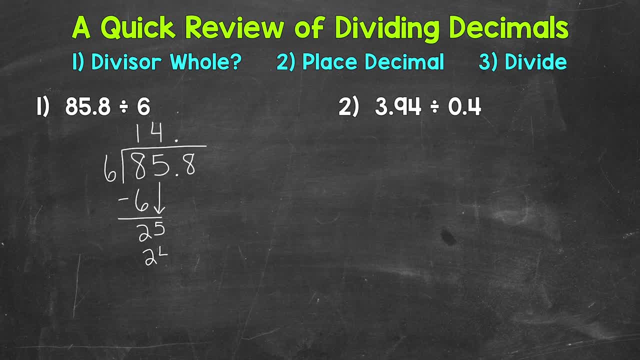 Multiply. 4 times 6, 24. Subtract. We get 1. And then, bring down our 8. 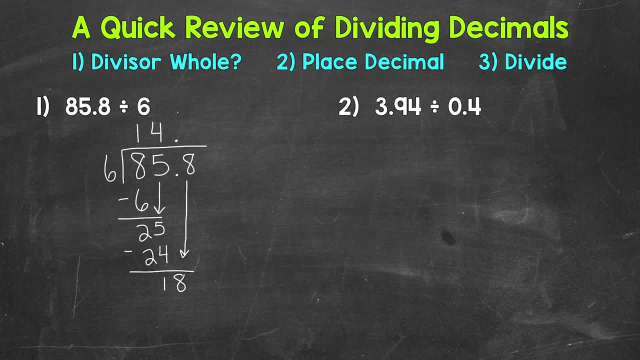 eight so we repeat now we go back to divide 18 divided by six how many whole groups of six in 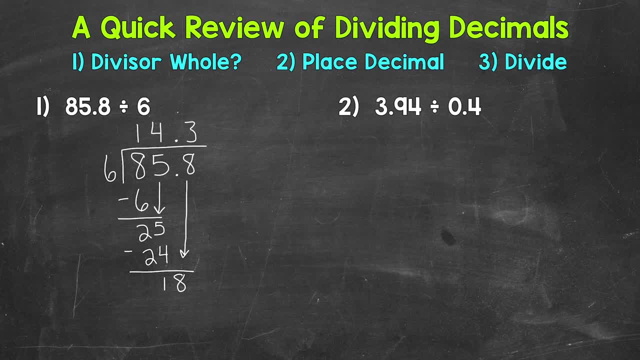 18 three multiply three times six is 18 subtract we get a nice clean cut zero there and we are 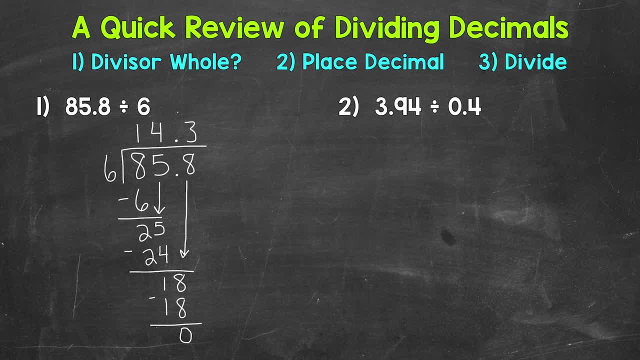 done we went all the way over to our furthest place value to the right in the case of number one that's going to be the tenths place and then we get that clean cut zero so we don't have anything left over we do not need to continue the problem now for number two we'll see what happens once we go all the way over and we do not get that zero there at the bottom once we subtract but for number one we are done our final answer 14 and three tenths let's move on to number two 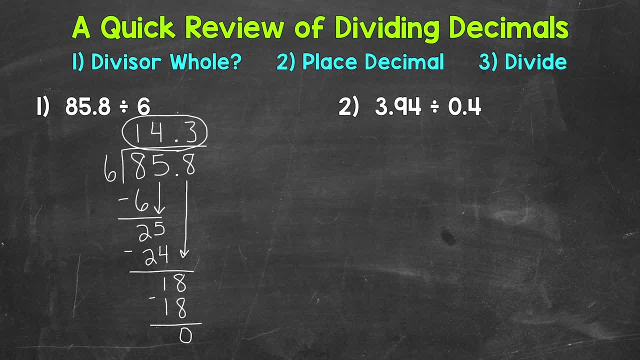 where we have three and 94 hundredths divided by four tenths so we need to set this up three and 94 hundredths is our dividend 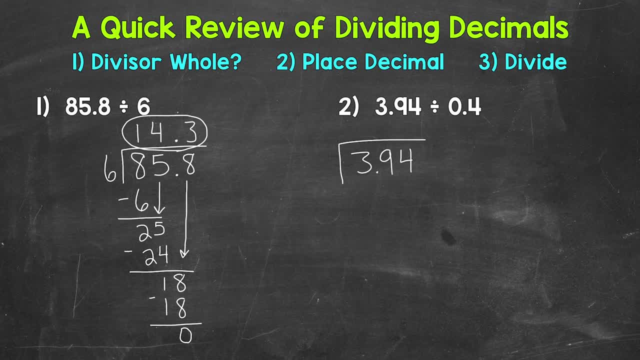 the number we are dividing and we are dividing by four tenths so once we're set up we need to see if our divisor is whole well four tenths is not a whole number so we cannot bring the decimal straight up quite yet if our divisor is not whole we need to make it whole making the divisor a whole number gives us the ability to go through our division steps and it's going to place our decimal for us in our answer it's pretty cool how this works out in order to make our divisor whole we need to move the decimal 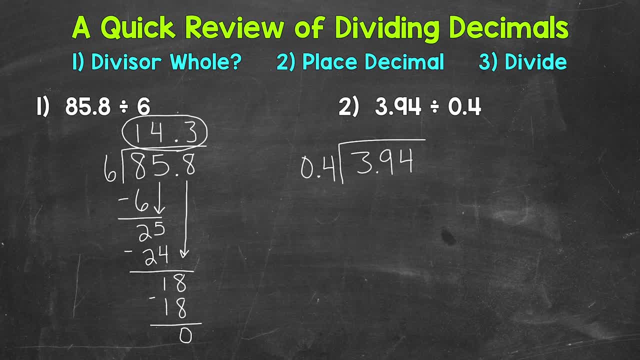 once to the right which means we are multiplying it by 10 so let's move this decimal once to the right 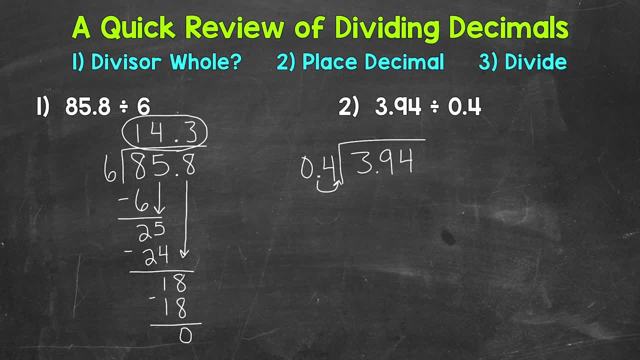 to keep this problem balanced, whatever we do to the outside, the divisor, we must do to the inside, the dividend. Again, this keeps the problem balanced and equivalent. Let's move the decimal once on the inside as well. So multiplying the dividend by 10 also. Once we get to this point, we need to rewrite the problem with the whole divisor and the decimal placed. So we have 4 for our divisor and then 39 and 4 tenths for our dividend. Now is our divisor whole? Yes. So we can bring our decimal straight up. Now it's placed where we need to have it in our answer and we can go through our division process. 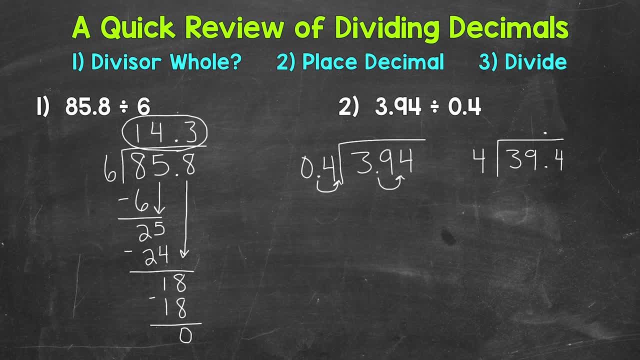 Now we start with divide. So we have 3 divided by 4. How many whole groups of 4 are in 3? Well, we can't do that. So we need to move over and use that 9 as well and work with 39. So we have 39 divided by 4. How many whole groups of 4 are in 39? Well, 9. That gets us to 36. 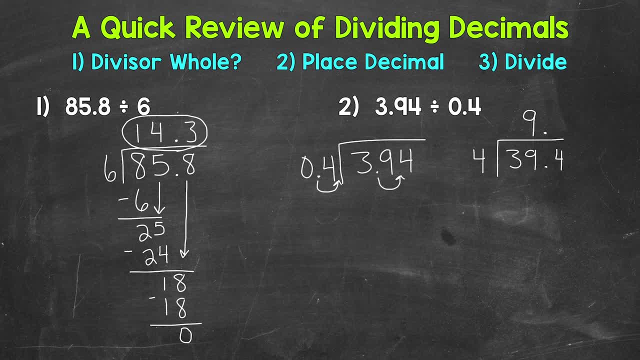 So let's write this 9 above the 39 there. Not above the 3. Make sure it goes above the 39. So we have 39 divided by 4. How many whole groups of 4 are in 39? Well, 9. That gets us to 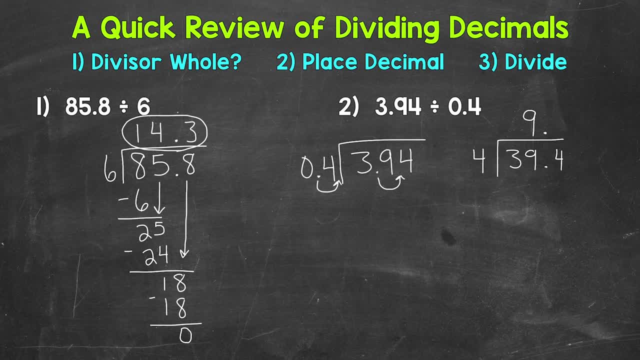 39. The 9 and 39 because we used both of those digits for our divide step. Now we multiply. So 9 times 4, 36. Subtract. We get 3. Then we bring down and repeat. So we have 34 divided by 4. How 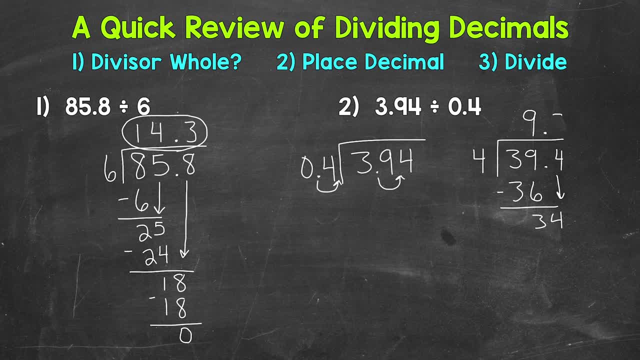 many whole groups of 4 are in 34? Well, 8. That gets us to 32. So 8 times 4 is 32. So we have 32. Subtract. We have 2. Now we went all the way over to the furthest place to the right. But we 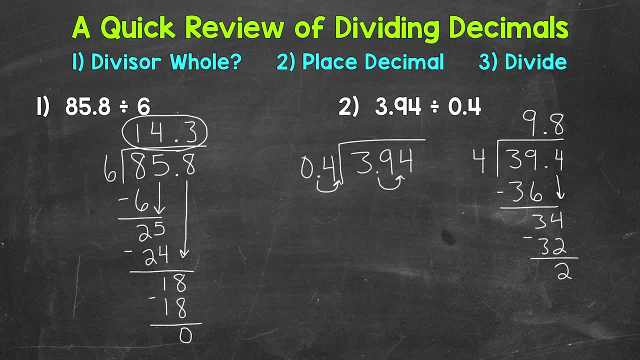 do not have a 0 at the end there once we subtracted. We do not want to put 9 and 8 tenths remainder 2. We want to keep this in decimal form for the whole problem. So what we need to do, we need to work until we get a clean cut 0. 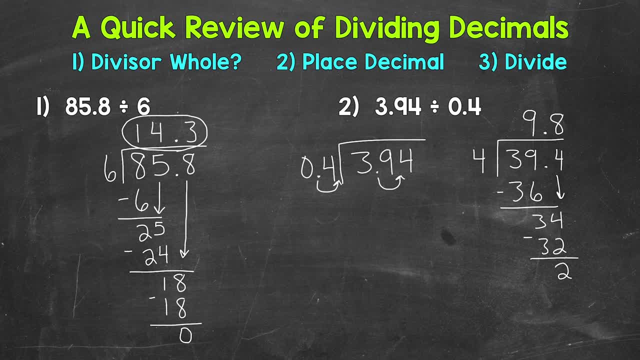 There at the end. And that's going to be our completed problem. So we need to put something on the end of this decimal to bring down and continue our process. So what can we put on the end of our 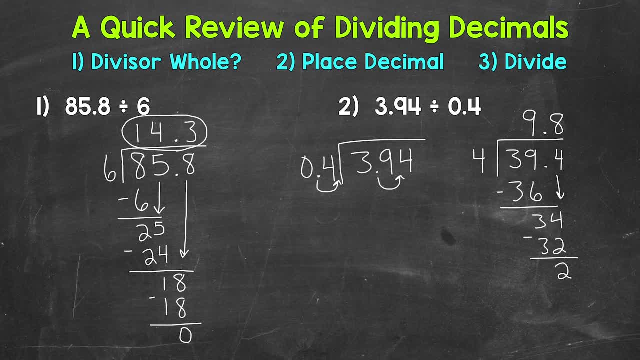 decimal that will not change the value of that decimal? Well, a 0. Remember, 0s to the right of decimal do not change the value of that decimal. So we can use a 0 here and bring that down in order to continue our process. So we brought down the 0. Now we repeat. We go back up 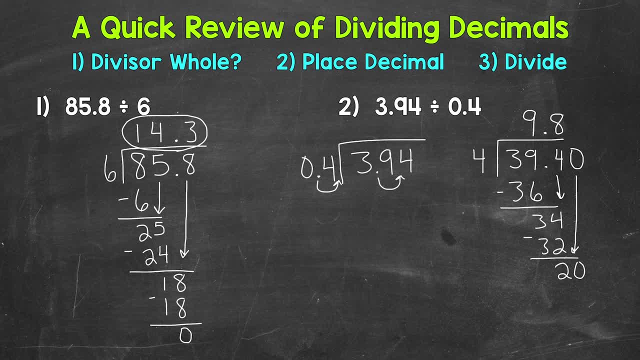 to divide. So we have 20 divided by 4. How many whole groups of 4 are in 20? Well, 5. That hits 20 exactly. And we can extend that bar there. Now we multiply. 5 times 4 is 20. And now we have that clean cut 0. We went all the way over. We needed to use a placeholder 0 in order to continue our process, which is perfectly fine. And then we worked to get that clean cut 0 and our final answer in decimal form. And that is going to be 9 and 85 hundredths. So there you have it. There's